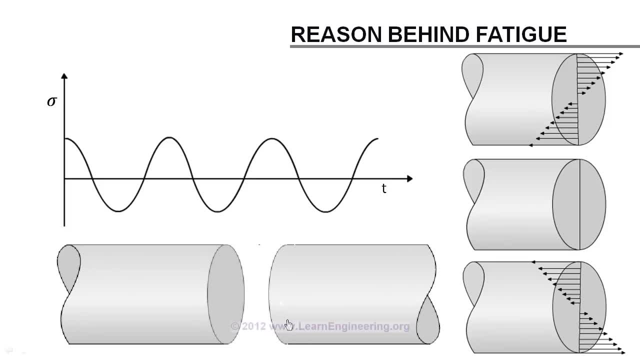 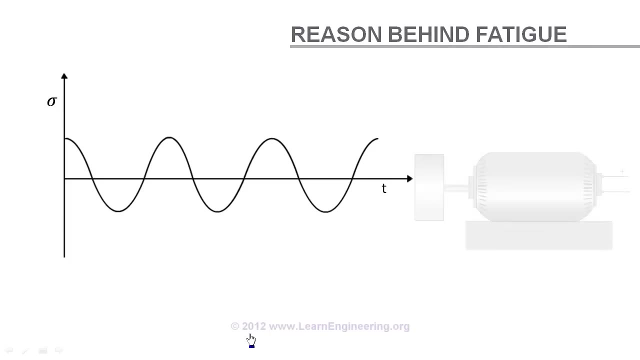 This is why failure due to fatigue is a dangerous affair, Unlike failure due to static load fatigue, failure happens without any warning. it doesn't even make a neck And the failure is completely unpredictable. The same phenomenon can happen for axle of this motor, where it is undergoing fluctuating stress due to gravity effect of this mass. 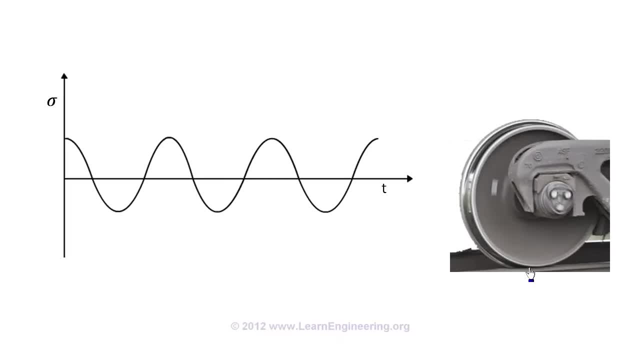 This rail wheel, when it is contact with with the track, produces a high contact stress. But when the wheel rotates, stress gets relieved. when it comes back to original position, contact stress arises again. So this also is a case of fluctuating stress. It may fail due to fatigue if we do not design it properly. 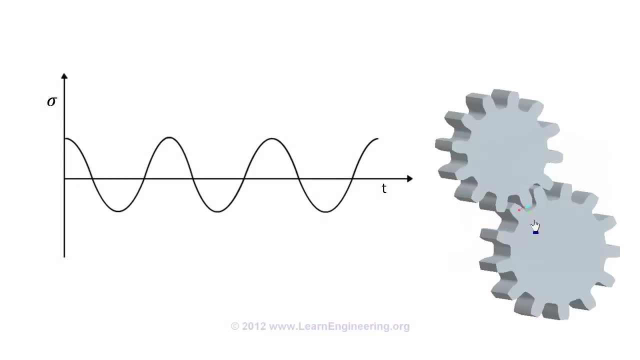 Same is the case with gear pair. Here, contact stress arises at mating point. Now the most important part in fatigue analysis: Relationship between stress amplitude and number of cycles it can execute before it fails. What will happen as stress amplitude decreases? Yes, you are right. as stress amplitude decreases, number of cycles required for failure increases. 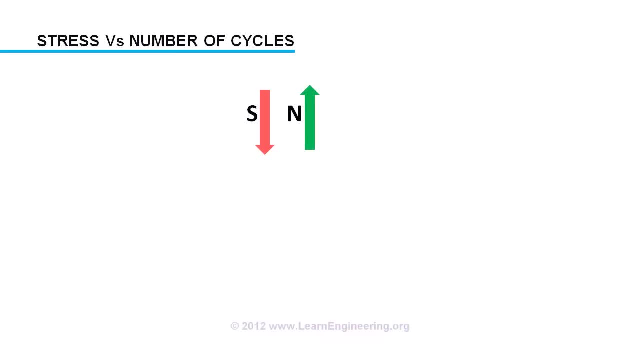 Anyway, we will analyze this trend more systematically. We will draw number of cycles in x-axis, stress amplitude in y-axis, Both in logarithmic scale. Let's start with the maximum stress a material can withstand its ultimate stress. So this will happen as you increase the stress, even before completing one cycle, the material will get broken. 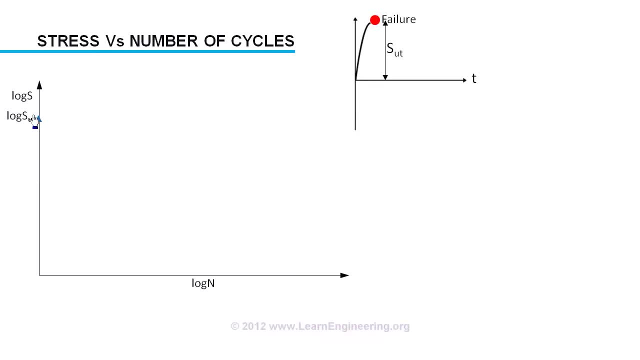 So this will be the corresponding point in SN graph. If you decrease the stress amplitude, it will execute more number of cycles before it fails. Decreasing stress even further, it will be able to execute even more number of cycles. So this will follow a trend like this. 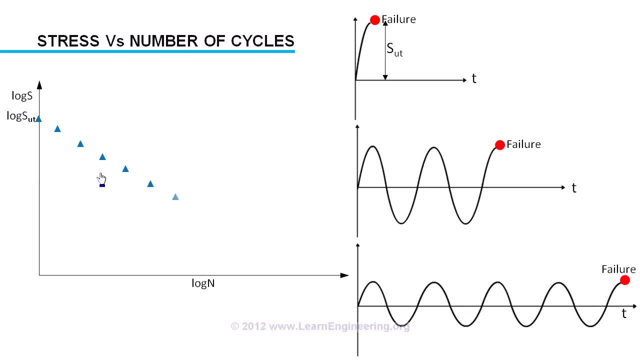 But not forever. You can see, after particular stress amplitude, even with slight decrease in stress, number of cycles required to make it fail increases drastically. Or, in short, if you have stress amplitude below this limit, number of cycles to make it fail jumps to infinity.